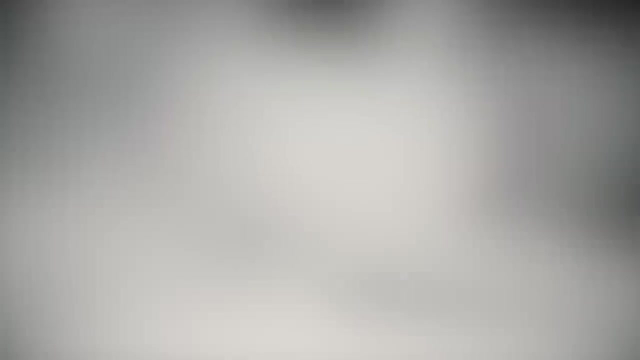 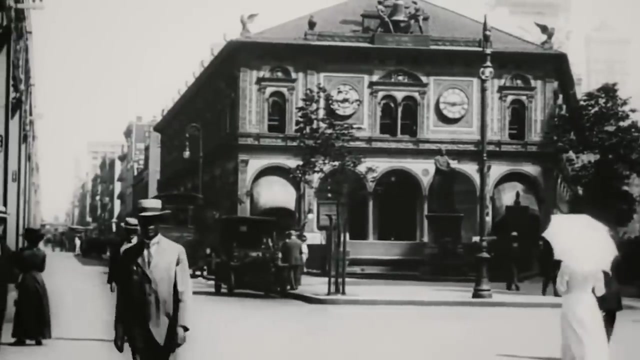 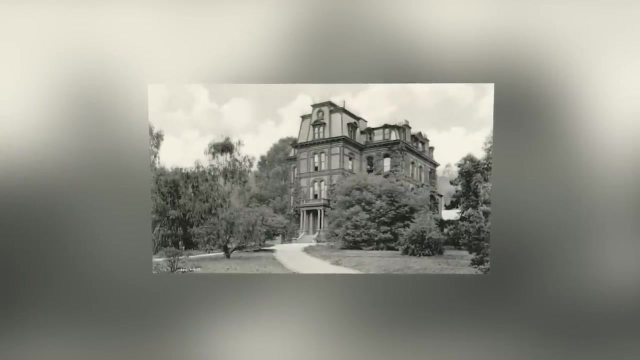 What's more is that George would often allow himself to skip class, which resulted in him being punished with extra homework. By the way, at this point we have approached our central point, one that can change your world view. So imagine the following scenario in the University of California in Berkeley in 1939.. 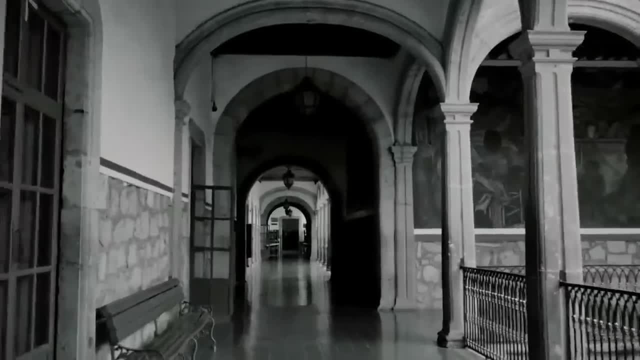 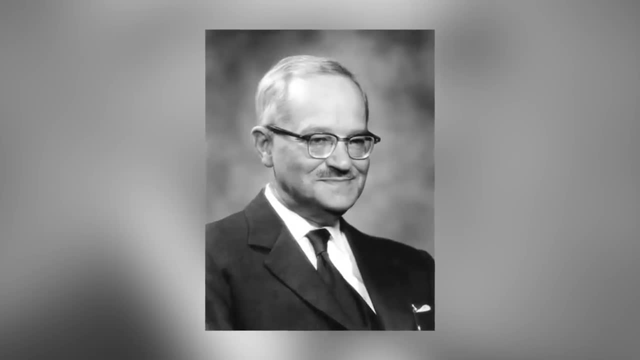 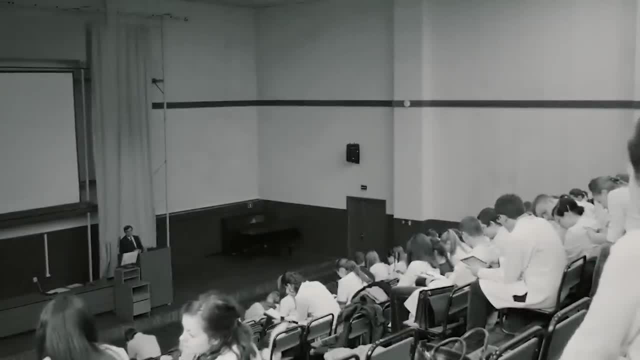 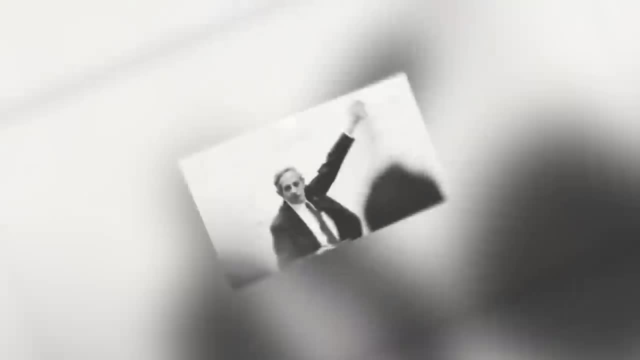 Having caught his breath only a little bit prior to entering the auditorium, he quietly opened the door and entered. The young man wanted to be unnoticed, so he sat down at a desk. quickly Afterwards he started looking around trying to figure out what he missed. 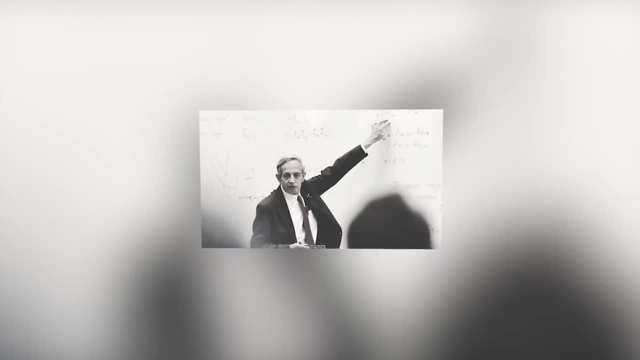 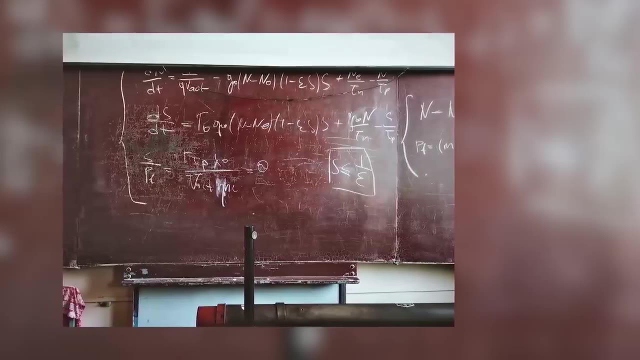 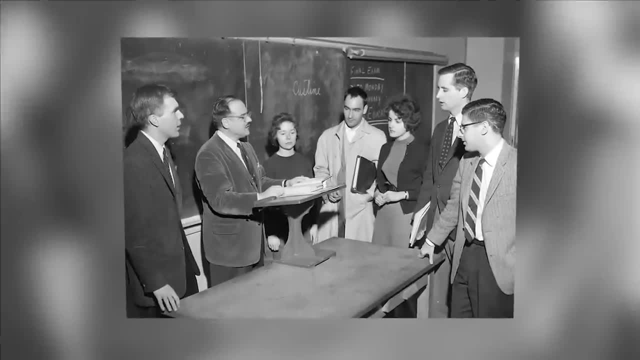 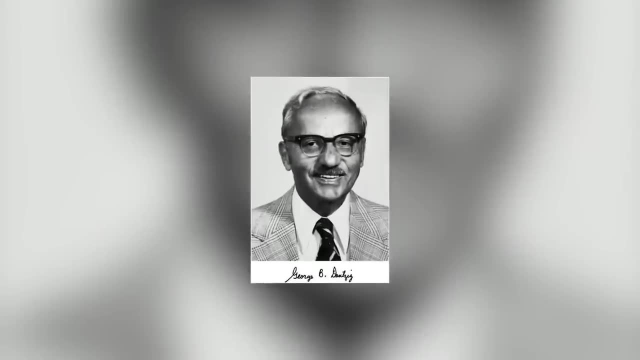 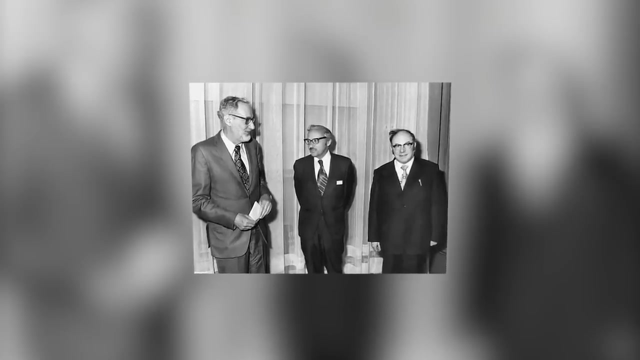 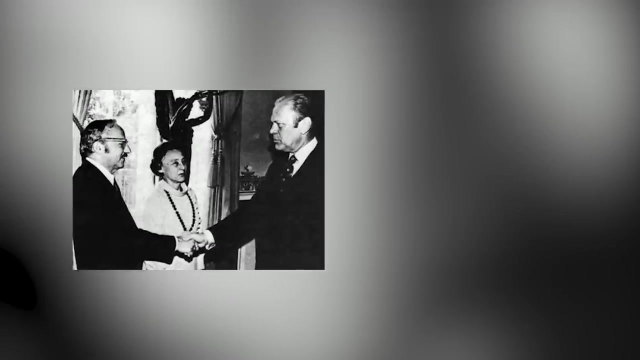 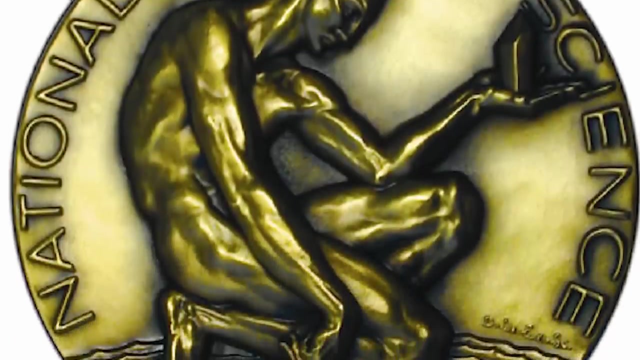 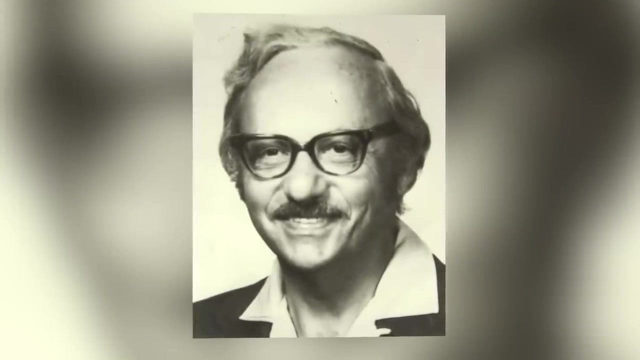 George thought that it was the next homework assignment for next class, so the irresponsible student simply gave up, James. Later, our student received the National Medal of Science and an honorary doctorate from the University of Maryland. In the 1970s he became a member of the National Academy of Sciences, the National Academy. 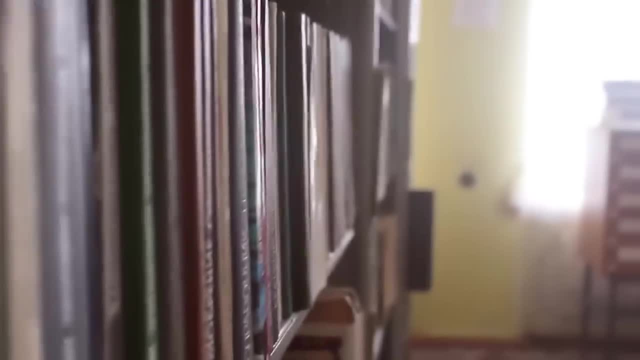 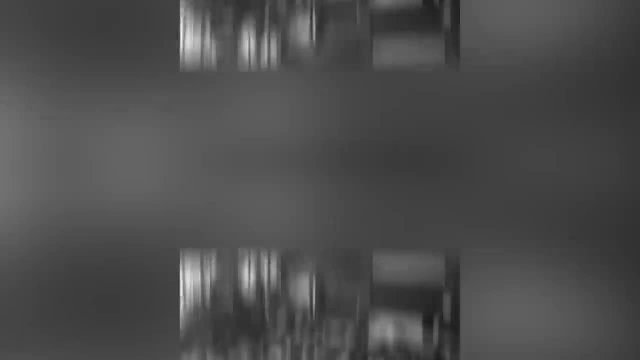 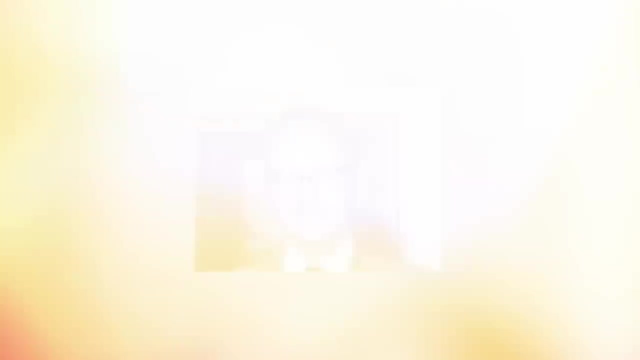 of Engineering and the American Academy of Arts and Sciences. He authored many papers and books. All this would have likely not happened and his name would not have been so widely known, had he come to that class on time. At least, that's what Professor George Danzig himself used to say with a smile.